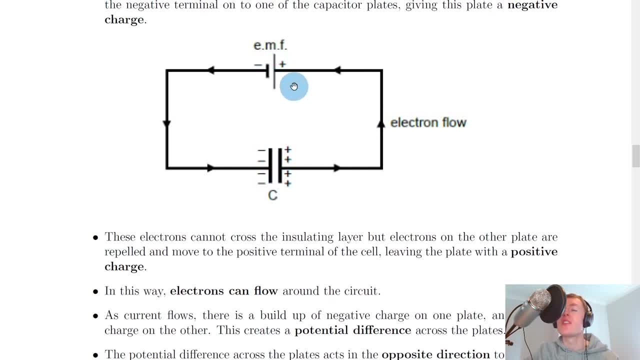 of the battery. But we're saying that if we've got a capacitor in the circuit, the electrons from the negative terminal are going to build up on one of the capacitor plates. So all of the electrons moving round in this direction will build up on this plate on the left hand. 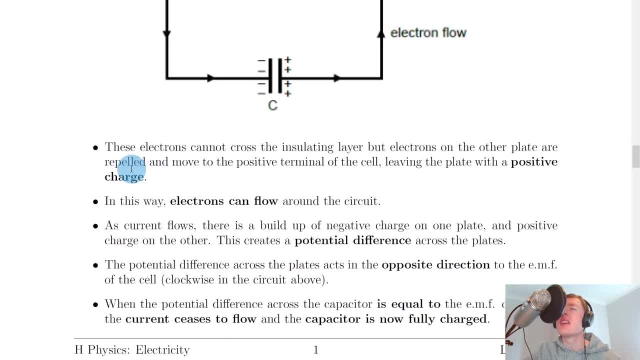 side here, Causing that plate to become negatively charged. It then says that these electrons cannot cross the insulating layer, but electrons on the other plate are repelled and move to the positive terminal of the cell, leaving the plate with a positive charge. 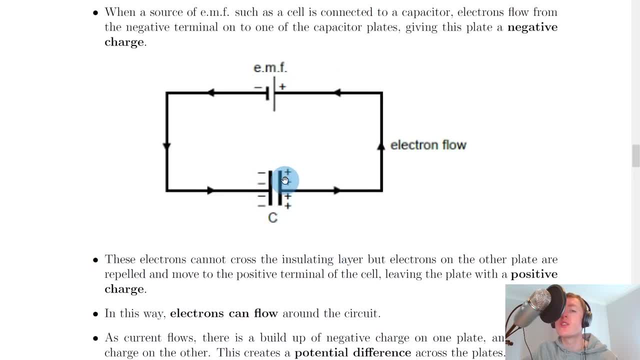 So the electrons on the right hand plate of the capacitor are going to be repelled away from the electrons on this side and they are going to move towards the positive terminal of the battery. And because these electrons have been repelled away, that means there is a net positive charge. 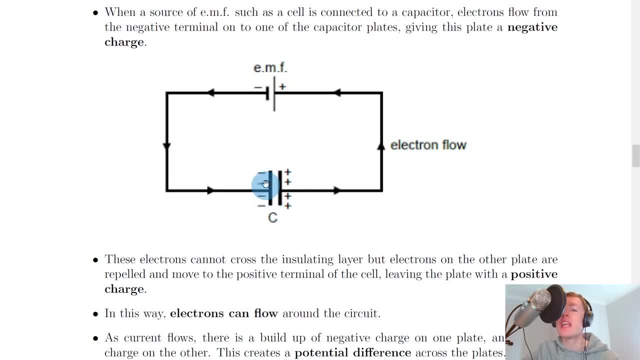 existing on this right hand plate of the capacitor. So we now have a negatively charged plate on the left and positive charge on this side left and a positively charged plate on the right, and this actually sets up an electric field and therefore a potential difference. So in this way electrons can flow around. 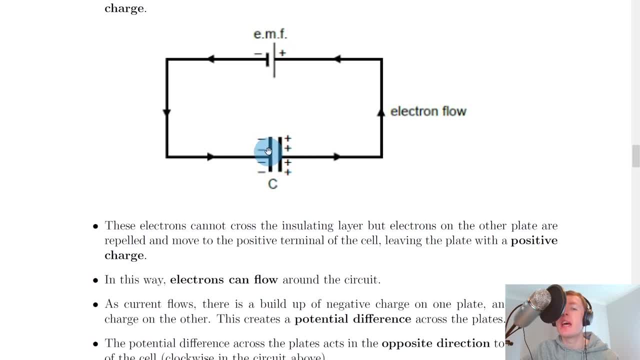 the circuit and we're saying that the electrons cannot actually cross the gap. it's the electrons over here that are repelling the electrons over here away from it, and in this way the electrons can continue to flow around the circuit As the current flows. there is a build up of negative charge on one plate and positive 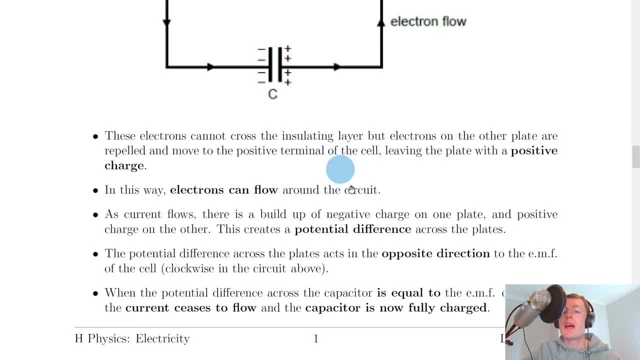 charge on the other. This creates a potential difference across the plates and this happens because of the electric field set up between the positively and negatively charged plates. So, remember, the electric field lines will go from positive to negative and the existence of the electric field creates a potential difference. 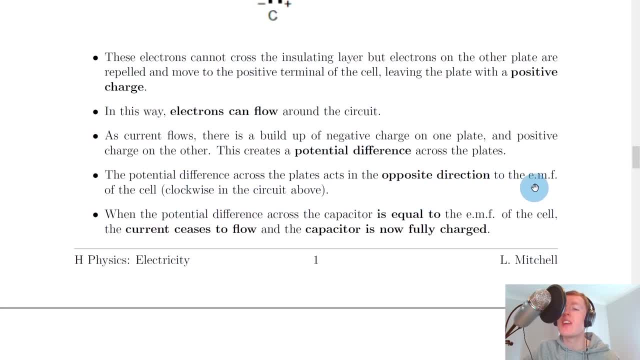 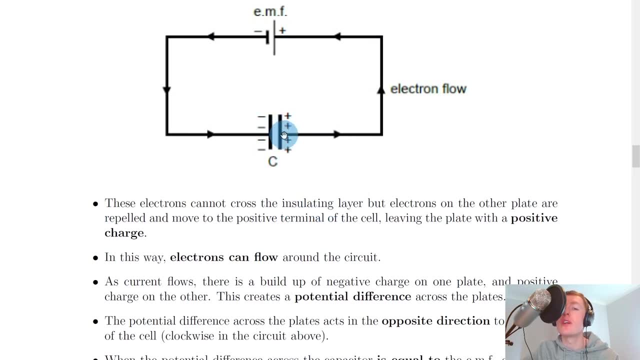 We say that the potential difference across the plates acts in the opposite direction to the EMF of the cell, ie clockwise in the circuit above. So all we're saying here is that the electric field direction is going to the left, in this case from positive to. 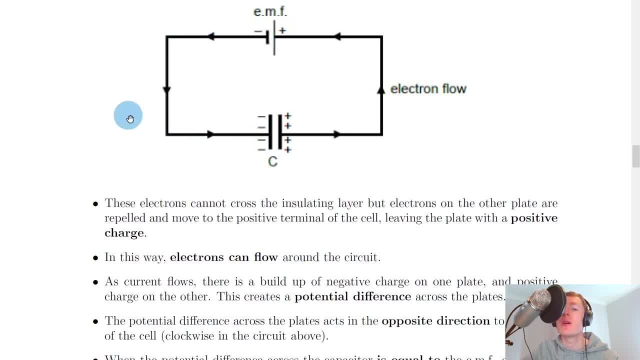 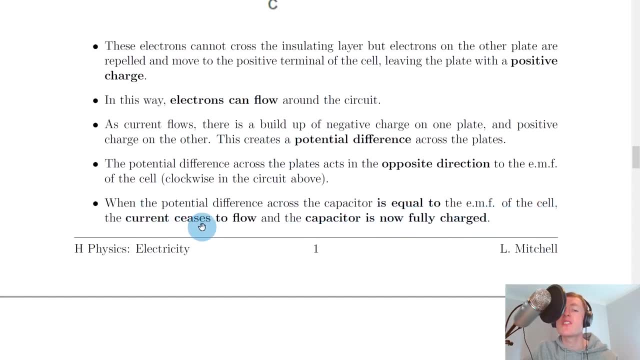 negative, and that is actually against the direction of the EMF, which comes anticlockwise here. Lastly, it says that when the potential difference across the capacitor is equal to the EMF of the cell, the current ceases to flow and the capacitor is now fully charged. Let's say we have a 10V battery. then when 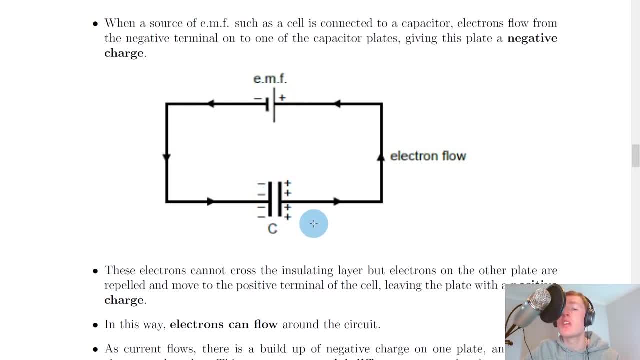 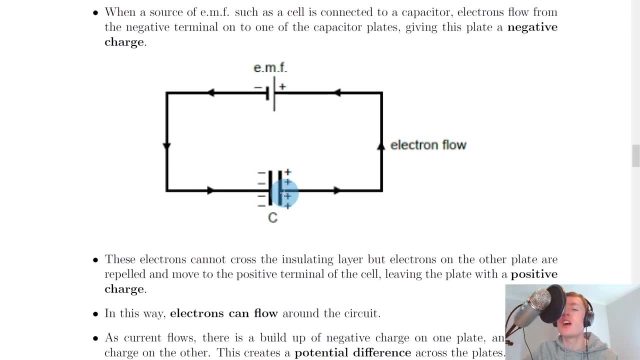 the potential difference across the capacitor increases to 10V, then we're saying that the current will stop flowing in the circuit and we say the capacitor is now fully charged. So the capacitor will be fully charged when the potential difference across it is equal.